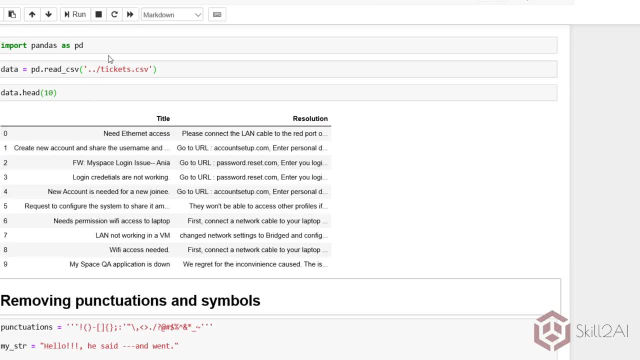 tickets data set. Now we can see that data set is here with title and the resolution. So whatever cleaning and pre-processing we will do, we will do on title because these are the possible classifications that we will be doing. So for now, let's see the cleaning. So in cleaning, 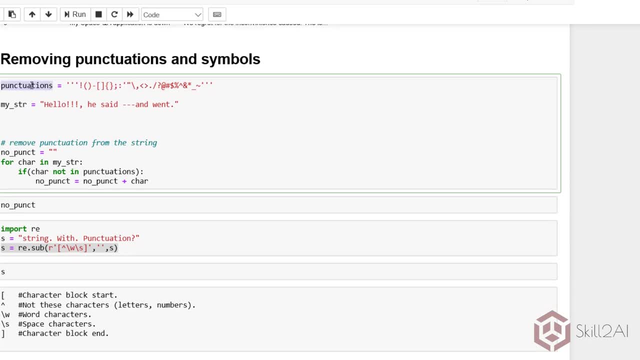 we remove the punctuations and symbols. So here I have taken a variable punctuations in which I have taken many symbols and punctuations, And I have taken a sample string for the demo case which holds punctuations and the string. So now, using a for loop, I can simply remove the punctuations from. 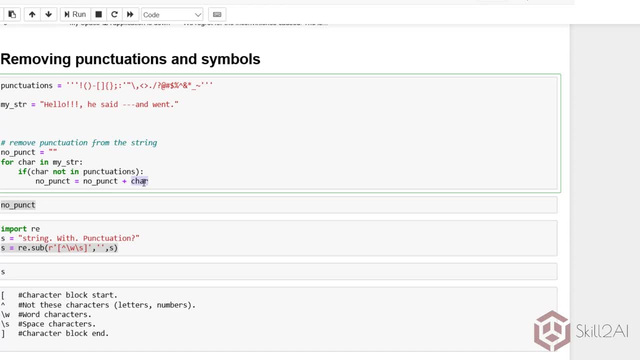 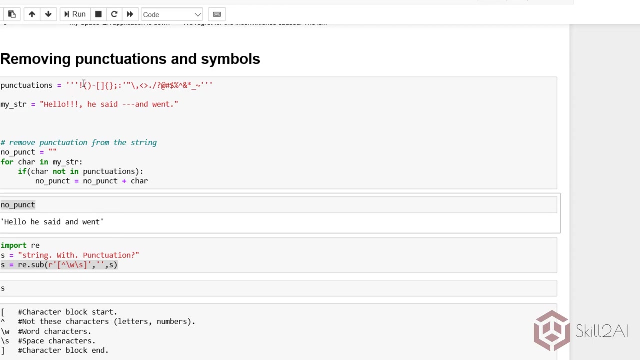 this string And then I can append the remaining characters to this newly defined variable, which is no punct, And it will. once I run this, you can see that it holds no punctuation marks. So let's see if I remove this exclamation mark here, so you can see that it will be. 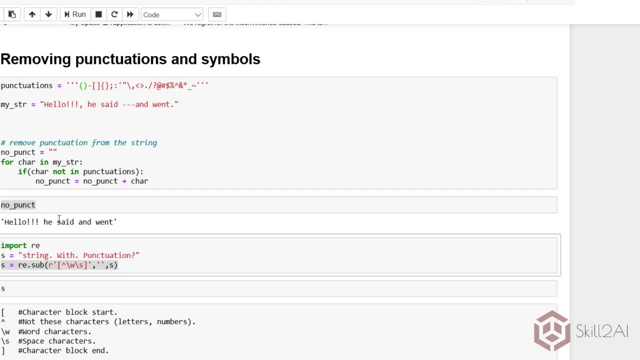 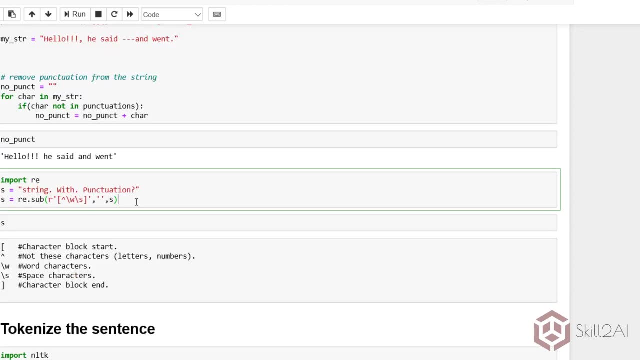 here also. So this is very simple and very weak Way of cleaning the symbols or punctuations. So the next thing to clean the data set is to use regex. Regex are based upon context, probably grammars, And if you see, I have assigned a variable, that string with punctuation, with the string. 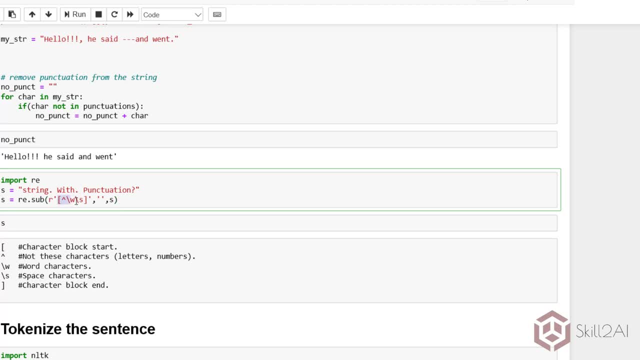 and then I'm doing a alert- is I have written a regex expression. so what is this regex expression? you can see it here. this symbol stands for not so after this, slash w stands for word characters and slash s stands for space characters. so this is how. this is a standard way of defining regex expressions. 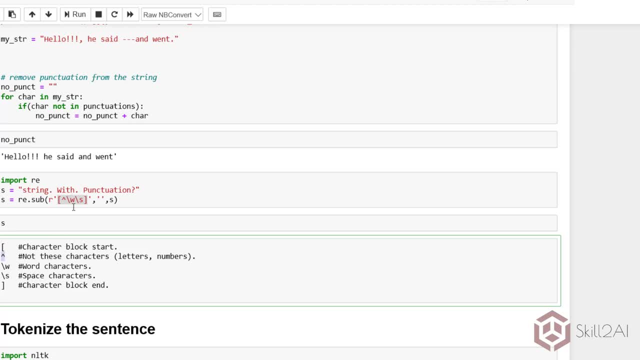 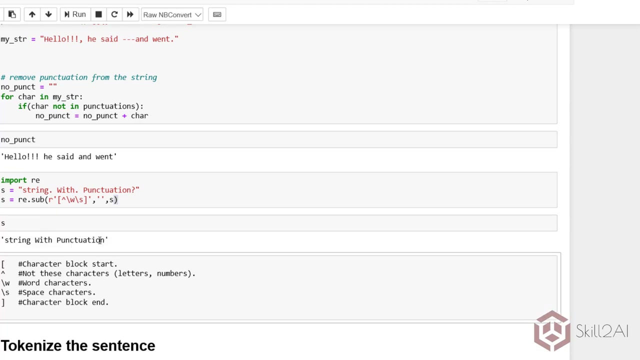 so it says a not of word characters and space characters it will not take, so this will not be selected. so what is going to happen is only with the space and the word characters are going to come in this regular expression, which is- and one thing to note, guys- that this regular expression 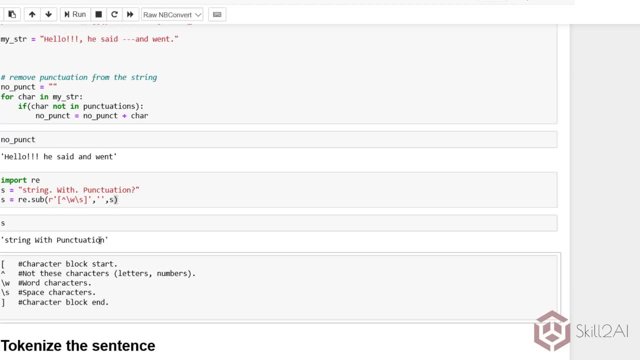 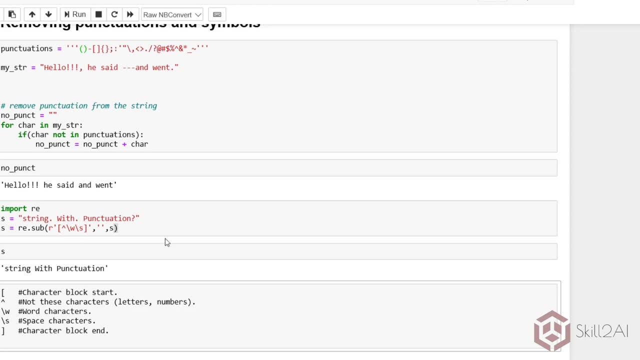 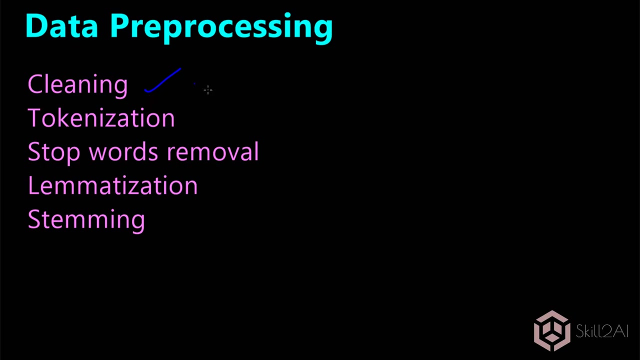 works very fast. so in very bigger data sets it is advisable that not to use this technique of like using for loop and going character by character, and instead using regular expressions. now the second step of data pre-processing is that tokenization. So tokenization is the breaking down of sentences into words. So because 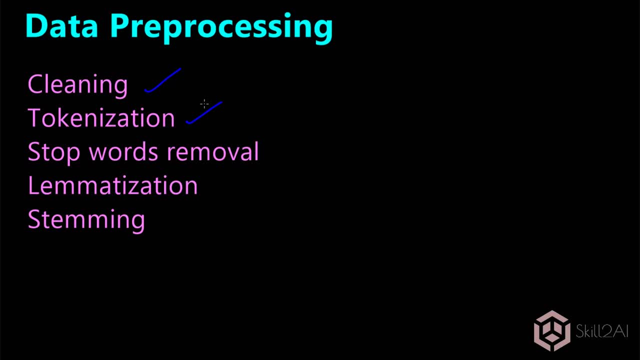 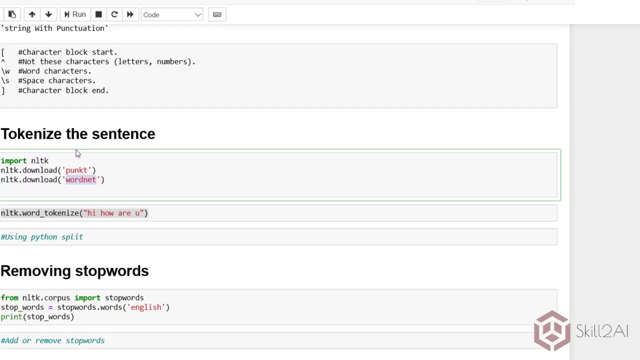 we need an individual meaningful entity to work upon and that in text can only be the words, right, it cannot be a character and it cannot be a complete sentence, but each individual words hold a meaning right. So let's see how can we do tokenization, So to tokenize a sentence we use. 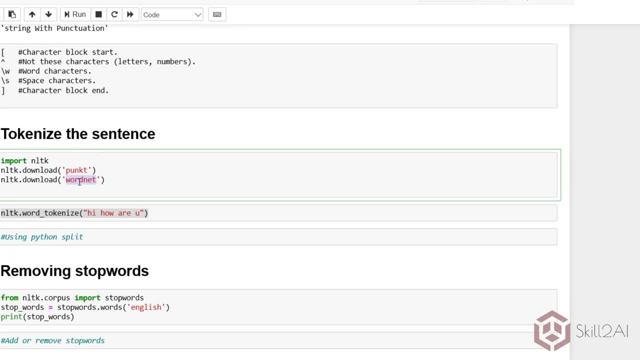 the NLTK library and it has some data dependencies which we can download using NLTKdownload punct and NLTKdownload wordnet, Because wordnet is the dependency of upcoming data pre-processing techniques but not the tokenization. So we can just simply use NLTKword underscore tokenize. 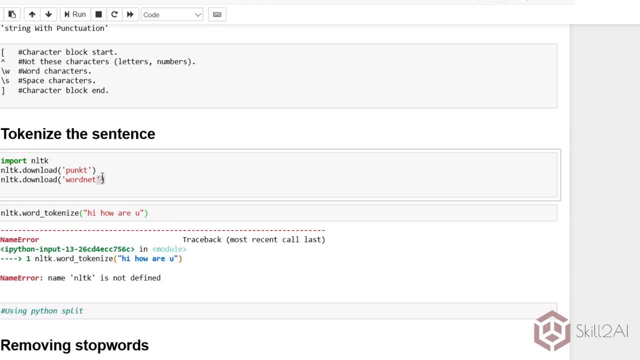 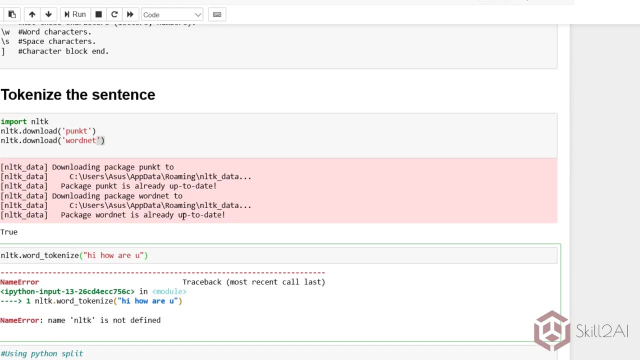 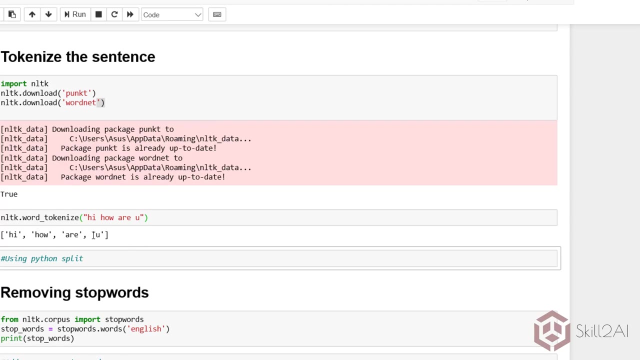 and if we pass the string, you can see. oh, first of all I have to run this and import the NLTK here. So now you can see it is being break down into a list of four words. Hi, how are you? So? this is the simple tokenization of a sentence which is used very much in the text pre-processing. 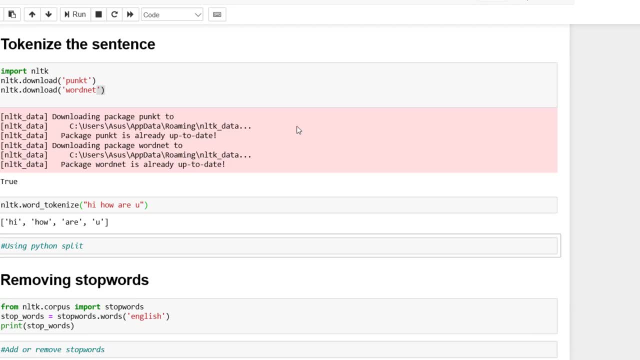 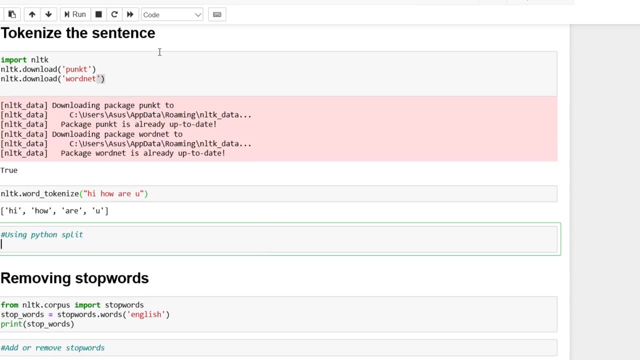 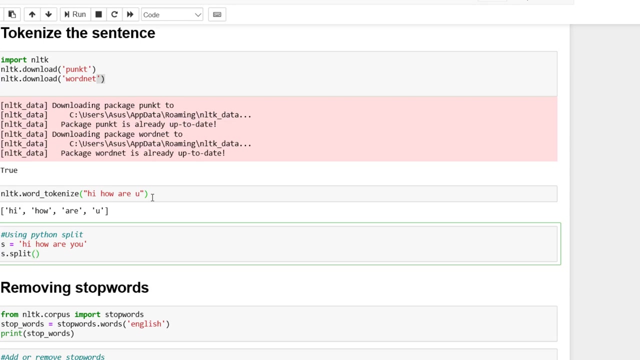 So we can also do it in other way, like using python split, Like: if I do s is equals to hi. how are you? and I do ssplit? You can see that the sentence has been broken down into words where we are using the space to split. So this also works, but it is advisable to use 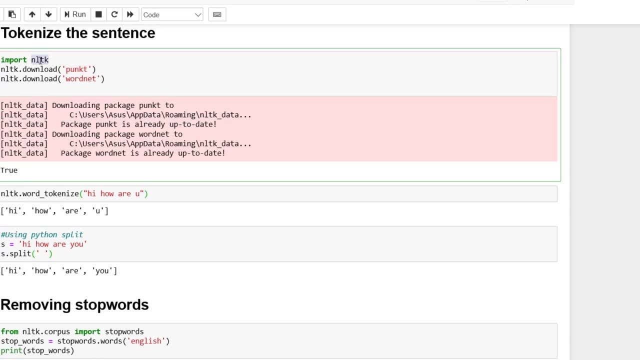 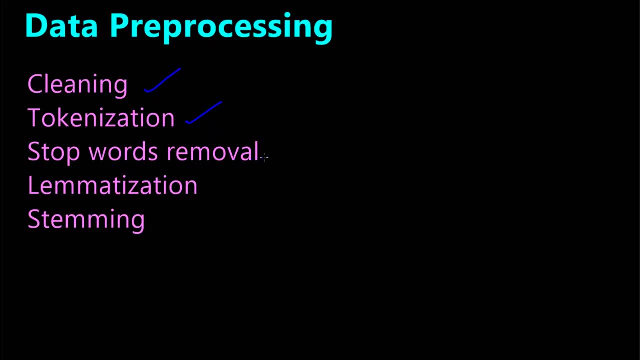 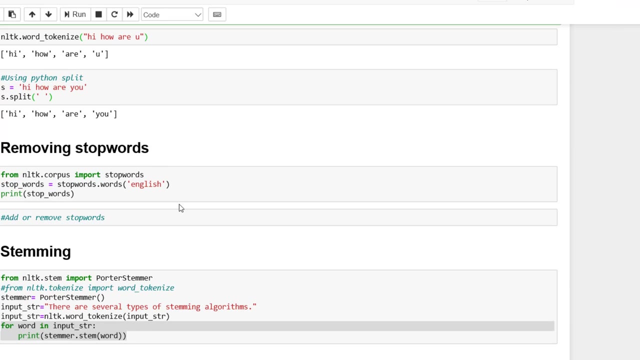 standard packages like NLTK, because these are better to use and very fast. Now the next step is to remove the stop words. So in stop words removal we again use NLTK and let's see what is a stop words and how to remove it. So stop words are those words which doesn't 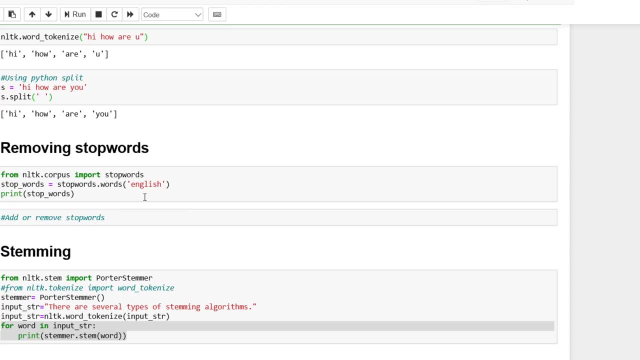 hold much value in the data set, just like I and or is did some determiners or conjunctions that don't hold much value, Right. These are not very important words. These are used very vaguely and in abundant. Right. It will be found across the data sets, in different data sets. 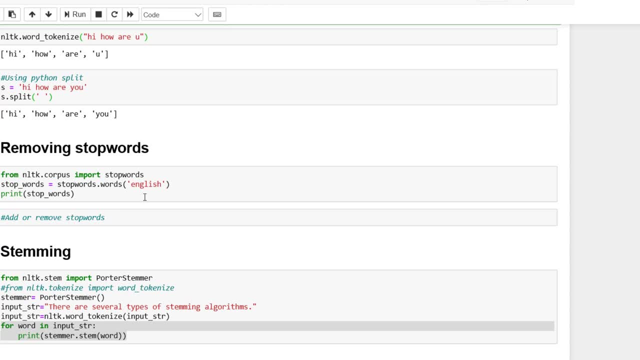 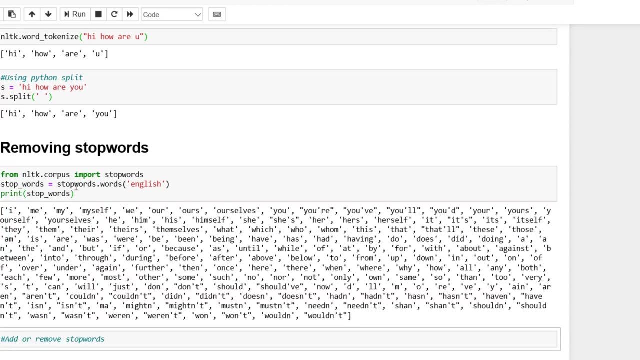 anywhere, because these are just basic determiners and used for the purpose of construction of the sentence, Right? So let's see, These are the stop words I'm talking about. I, me myself, we are ourselves. So these don't hold much value or much meaning to the sentence. So 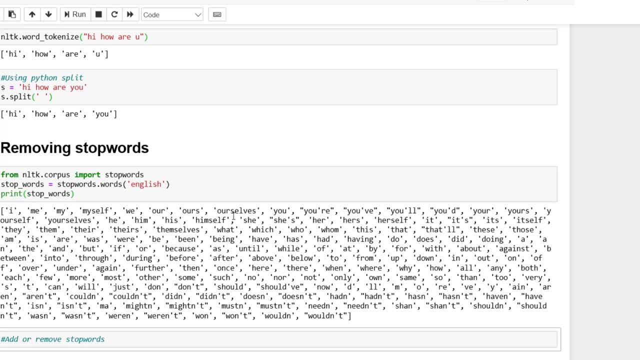 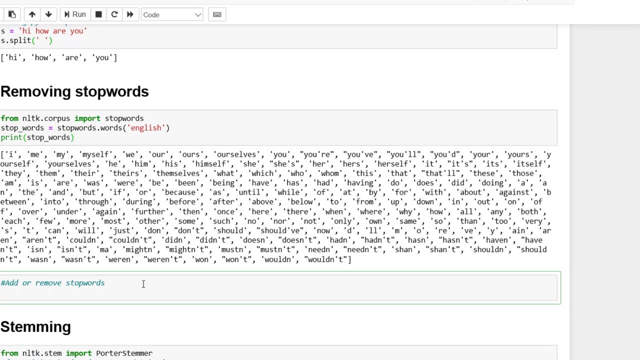 that's why, Sometimes, What we do, We remove the stop words from the data set. So if we want to add or remove stop words, we can also do it like this, because it's just a list, So if we append to the list, 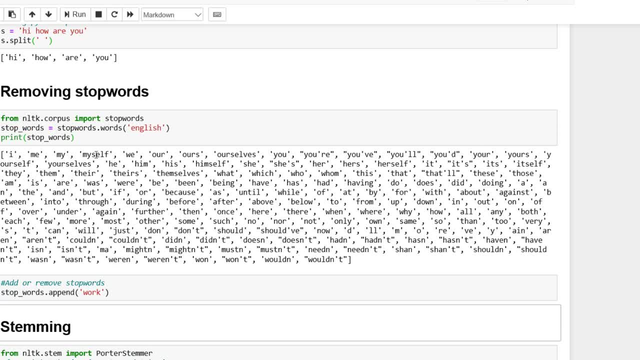 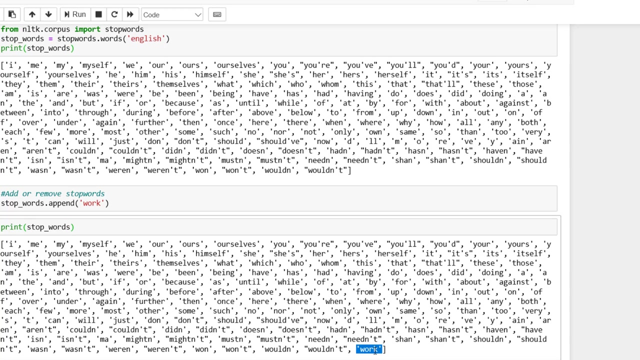 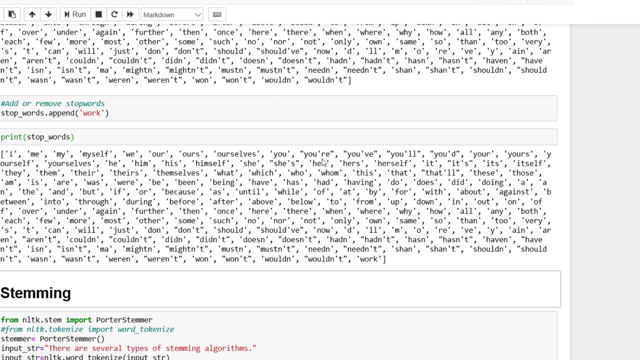 it will work Right. As I'll say: work right now. Now, if I again print the stop words, You can see that work has been added. So in the similar fashion, you can remove or add the stop words which we have imported from the NLTK corpus. Now to remove the stop words. 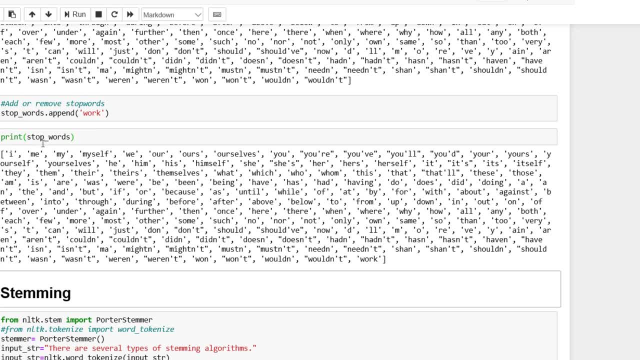 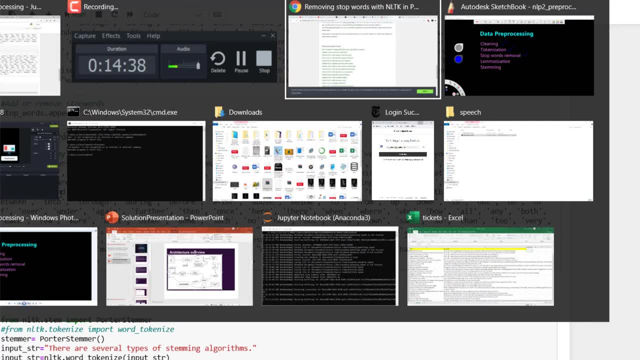 you can iterate over each word in the sentence and see if that word is present in the list or not and then remove it. So the next step In the data pre-processing is the lemmatization and stemming. So I will come to the lemmatization. 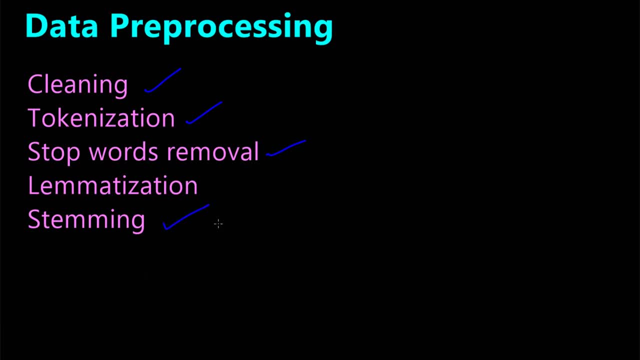 in a while, and before that I will explain the stemming. So stemming is simply to reduce the words to their word stems- See, just like we have a word males, See male. if we stem, if we use stemming, we can chop off the word from here and the reduced form of word will. 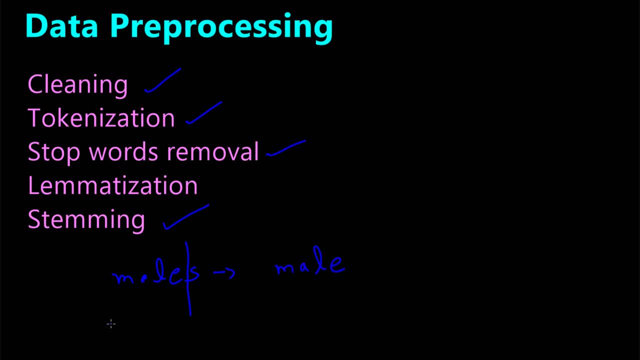 be male Likewise. Likewise, if I say another word, playing, and I stem this word from here, it will become play. So sometimes these kind of words become a standard and we use stemming because it is very simple to use, because if we don't do this, then this males and male will be two. 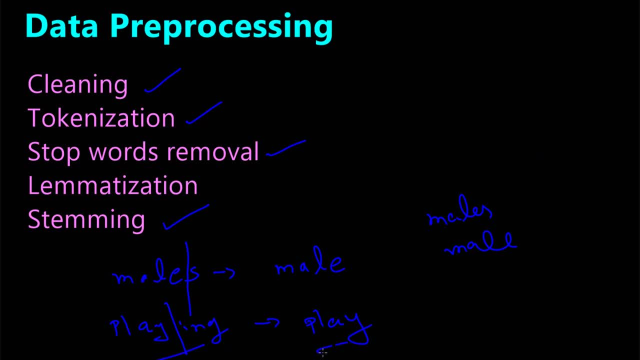 different words. Right, Simply this, playing and play will be two different words. But if we use stemming, then we can resolve this playing to play. Then again our algorithms, or whatever we are using, can be able to detect that this play is the same play that we were. 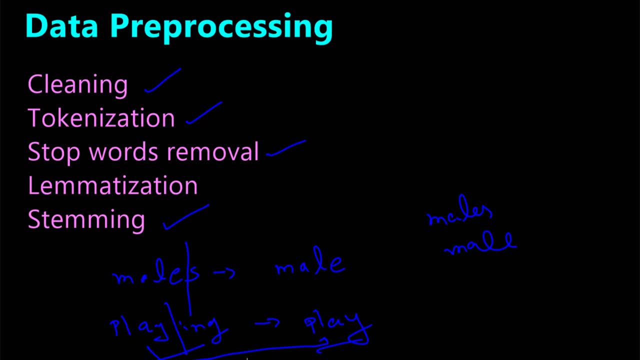